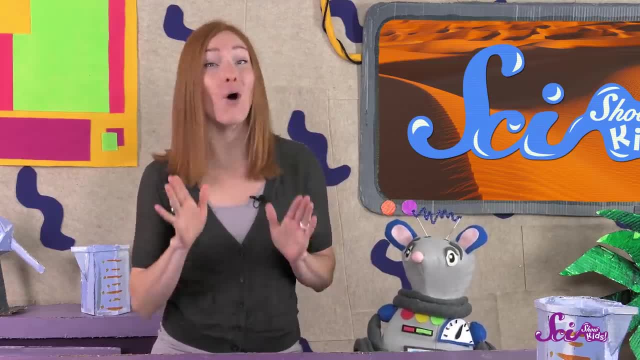 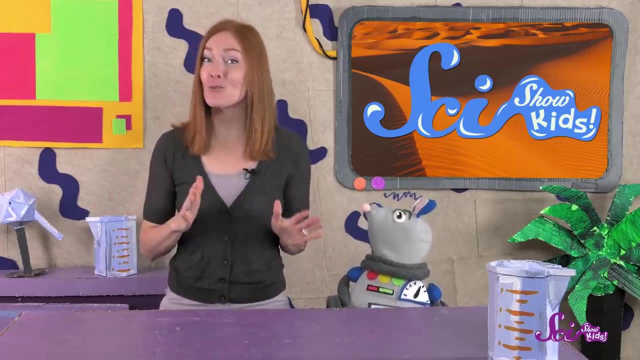 In deserts there's so little rain that sometimes you have to wait a whole year just for one rainstorm. So things that live in the desert, like plants and animals, and even people, need special ways to survive when there's so little water. 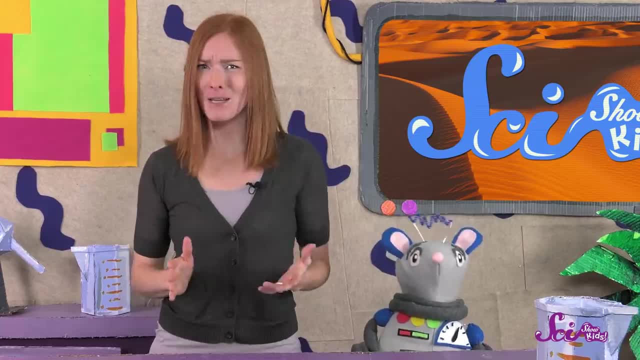 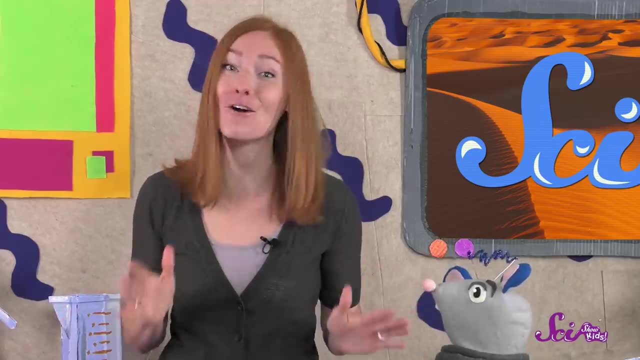 They also need special ways to deal with the temperature in deserts, because deserts aren't just very dry, they can also be very hot or very cold. Hot deserts are the kind of deserts you might have heard about before. They're incredibly hot, just as hot as the middle of the summer all year, though they 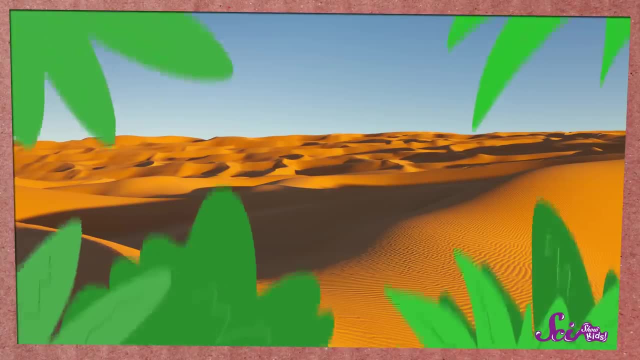 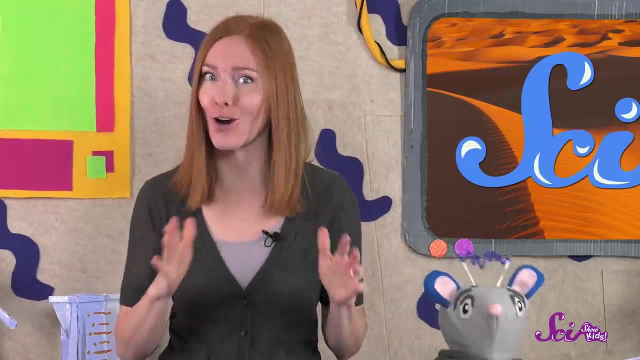 can also get pretty chilly at night. Hot deserts don't have a lot of big leafy plants that can help provide shade during the day or anything to hold in the heat at night like a blanket. But not all deserts are hot. 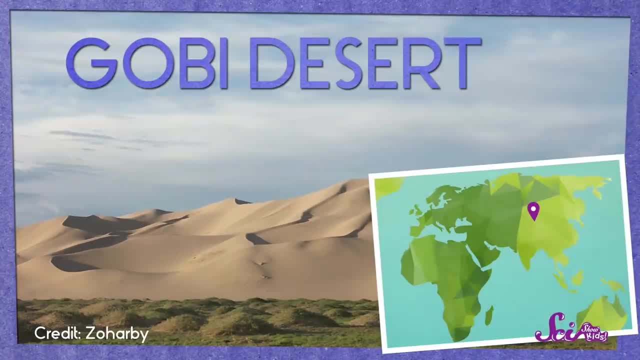 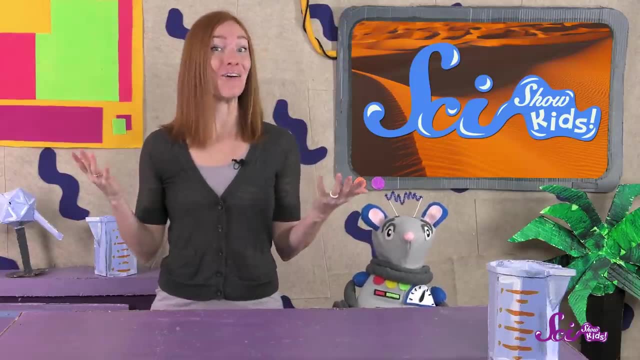 There are actually cold deserts too. During the summer, cold deserts aren't too cold, but when it gets to be winter, they're freezing. When you think of the cold, you might think of snow, But it hardly ever snows in cold deserts, even though it's so cold. 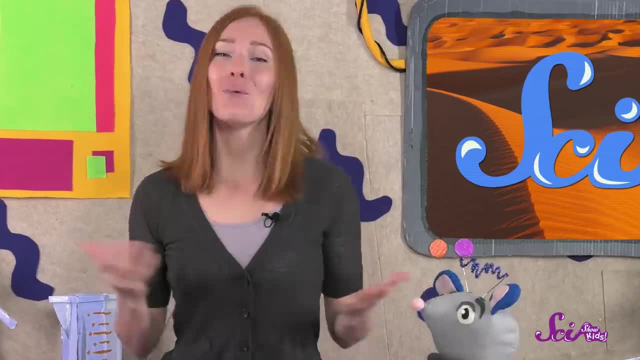 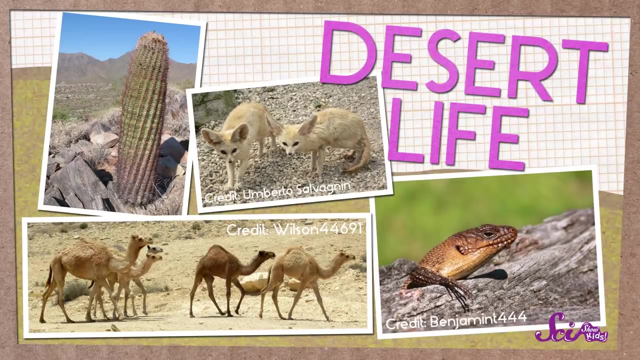 There might only be a tiny bit of snow or rain all year. Whether their desert is hot or cold, all the plants and animals that live in deserts have to be really well-prepared to live in such an extreme place. One of the main things that's hard about life in the desert is that they're so cold. 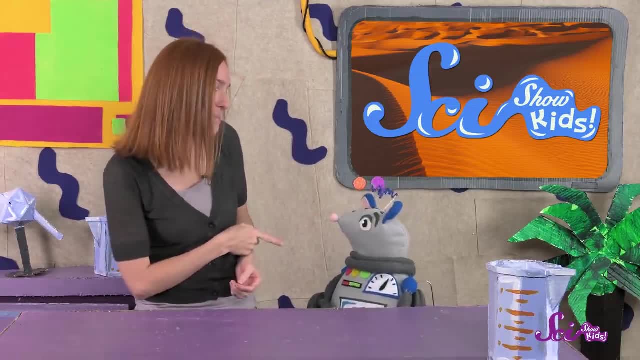 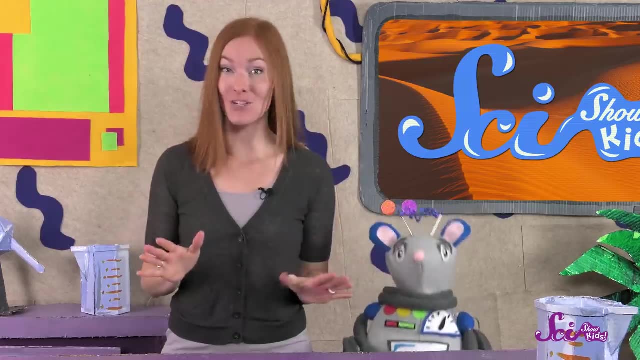 There's so little water, So Squeaks. what do you think plants or animals can do to make sure they have enough water? That's right. Some of them have special ways to hold onto whatever water they can find, Like a cactus. 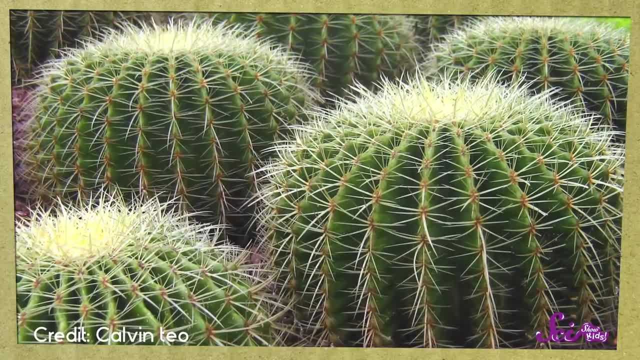 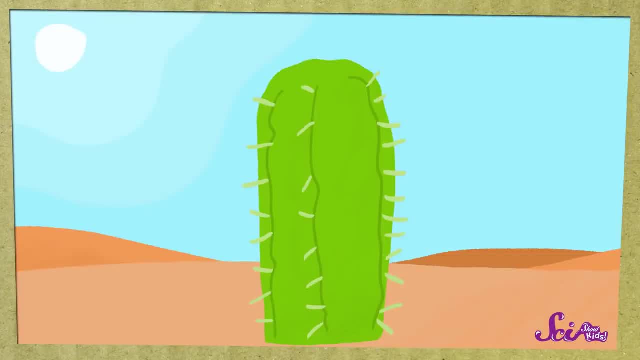 Cactuses are plants that live in deserts, and they have thick stems where they can store water for a long time. It's almost like they have a water bottle built into their bodies. So, even though it doesn't rain very much, whenever it does rain a cactus will soak. 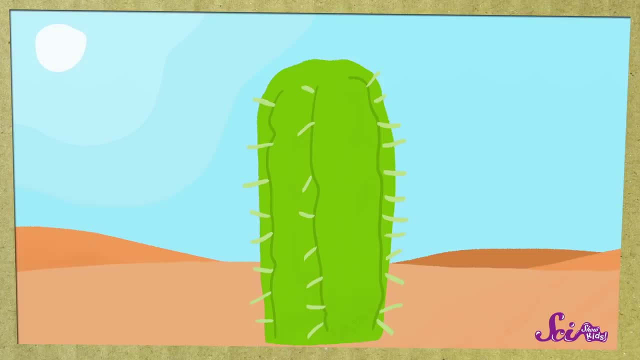 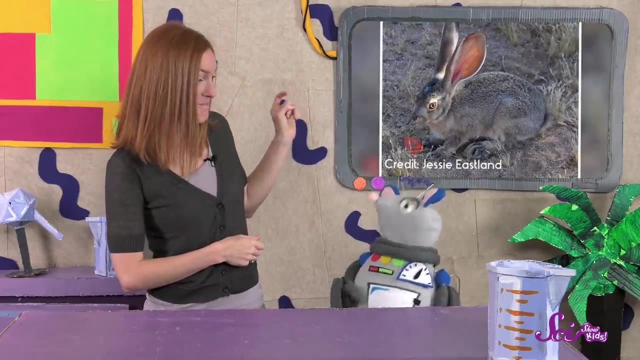 up lots of water and save it, So it has water until the next time it rains. But that's not the only way to get water. when it hardly ever rains- Squeaks. do you know what kind of animal this is? You're almost right. It does look a lot like a bunny rabbit, but this is actually a different kind of animal called a jackrabbit. Jackrabbits live in hot deserts in the United States and Mexico, and they mainly get their water from the plants they eat. They also do something kind of funny to make sure they get as much water as they can. They eat their poop. Anyway, they can get any water that might have been left in it. The other thing that's really hard about living in a hot desert is that it's sohot. 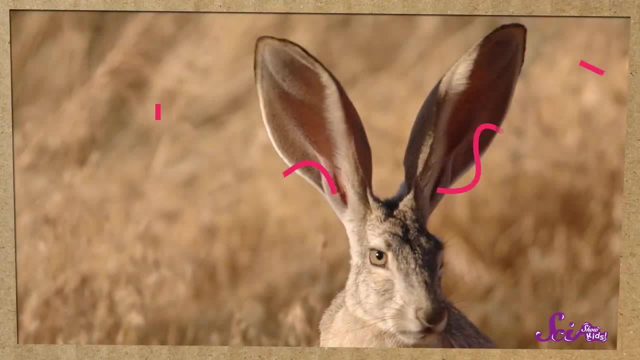 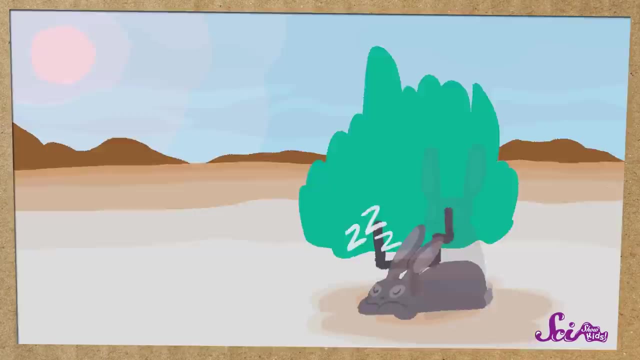 That's why jackrabbits have those huge ears. They're big, so the jackrabbit can cool off really quickly. Also, jackrabbits don't do much during the day, when it's the hottest, They sleep instead. They're mainly active early in the morning and in the evening, when the sun isn't as 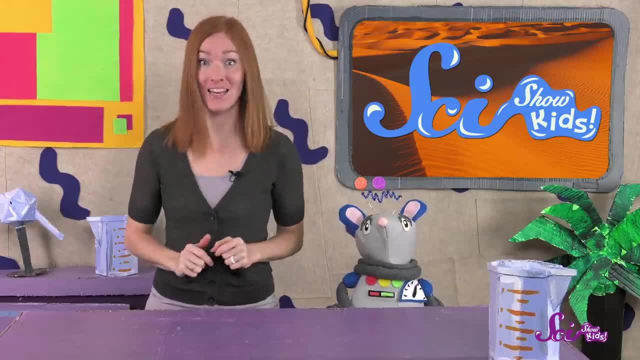 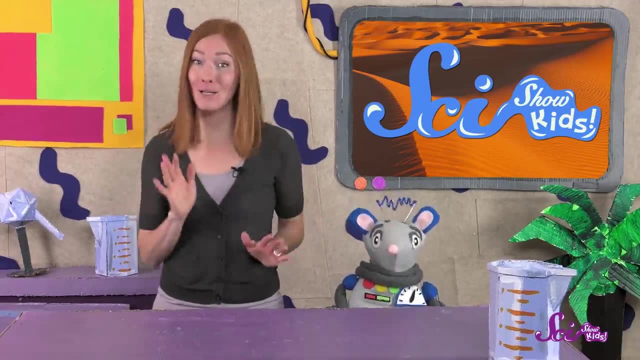 high in the sky and it's a little cooler. They're also active at night. But what about animals that can choose to live wherever they want, like humans? Well, people have lived in deserts for an incredibly long time and we've come up. 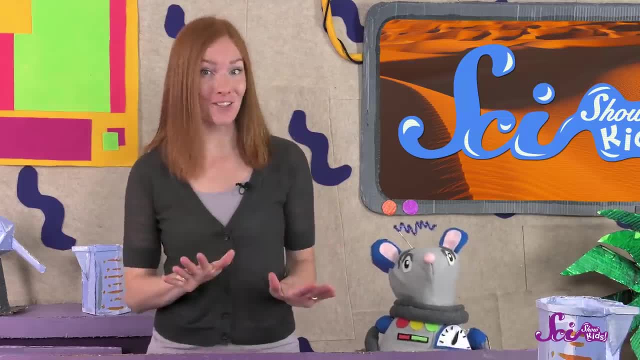 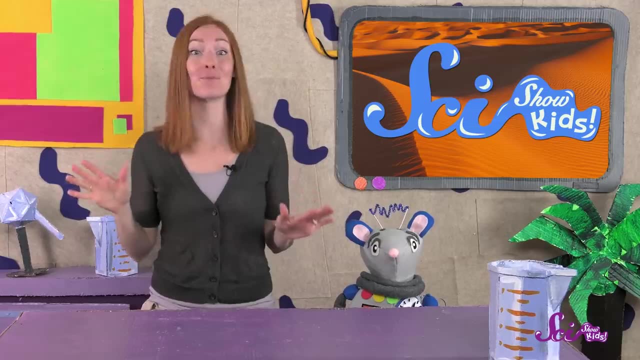 with all kinds of ways to survive there, But some humans live in the desert, using some of the same tricks as other animals that live there. People who live in deserts can choose to wear special loose clothes that allow the breeze to cool them off. 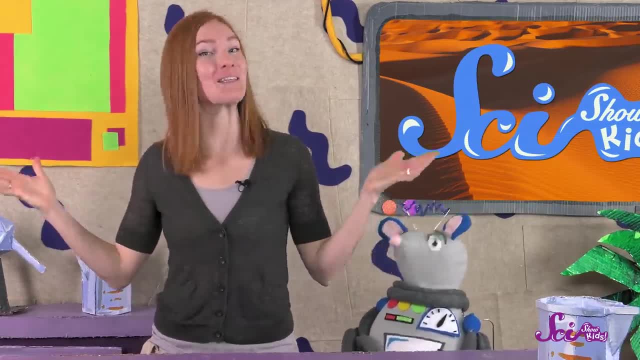 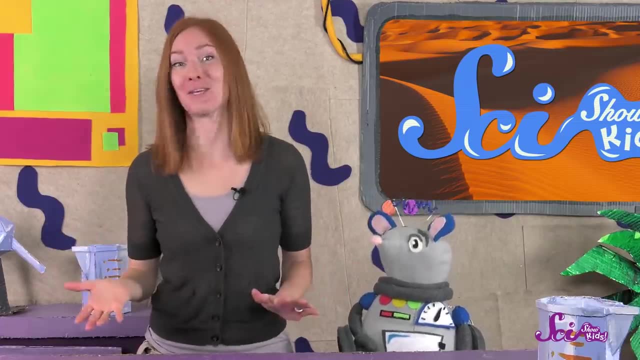 These clothes work a lot like a jackrabbit's ears, letting people catch a breeze and cool off quickly. People also have to avoid the intense heat of the hot desert sun. You could try bringing an air conditioner with you wherever you go, but some people use it to keep them cool. They only go out when the sun is low. Just like many desert animals, some people will wake up early, when the sun is just rising, and get things done in the morning. Then, during the hottest part of the day, they'll rest in the shade. 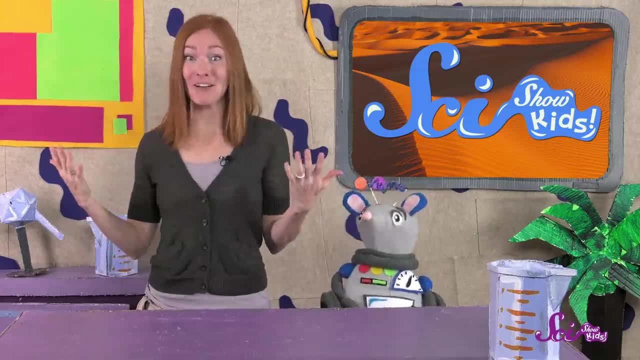 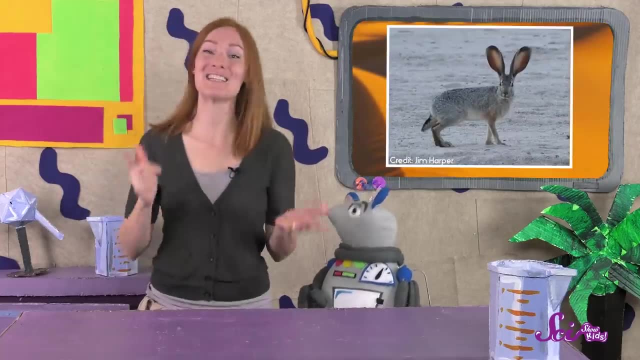 And then, once the sun is setting, the air gets cooler and everyone can go outside again without getting too hot Squeaks. do you remember which animal also does this? That's right, Jackrabbits are active in the mornings and evenings too. And there are lots of other desert animals that live this way too, Like this one, Like coyotes, birds and even porcupines. Animals that are most active at sunrise and sunset are called crepuscular, And it turns out that being crepuscular is a pretty good lifestyle for people in the 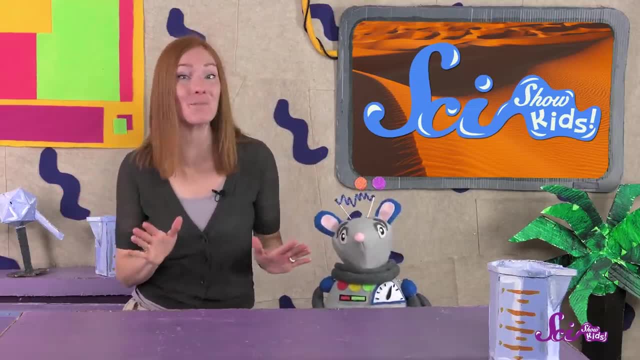 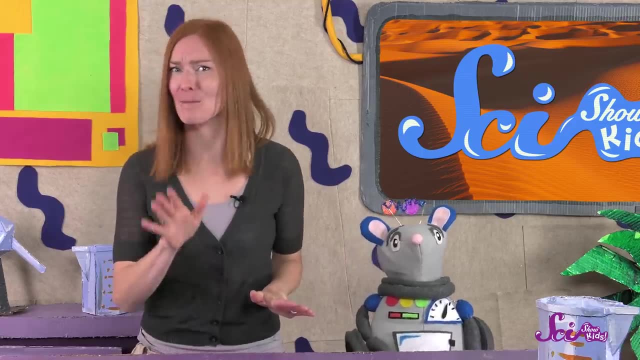 desert too. There are so many interesting ways to live, even in a place as dry as a desert. No matter how they choose to do it, the people, other animals and plants that live in deserts have to be pretty tough. 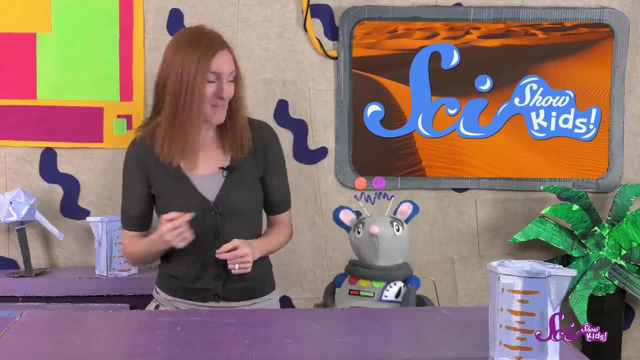 Thanks for joining us on SciShow Kids. If you want to keep learning and having fun with me and Squeaks, be sure to click the red subscribe button. Thanks, and we'll see you next time here at the Fort. 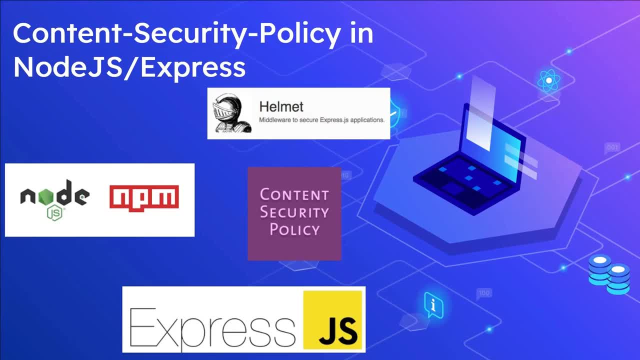 Hi all, welcome to tech forum. In this video let us see how to enable content security policy headers in express js applications. In our earlier video we have seen what is content security policy headers and how to use the CSP headers to protect the websites. The CSP headers instruct the client. 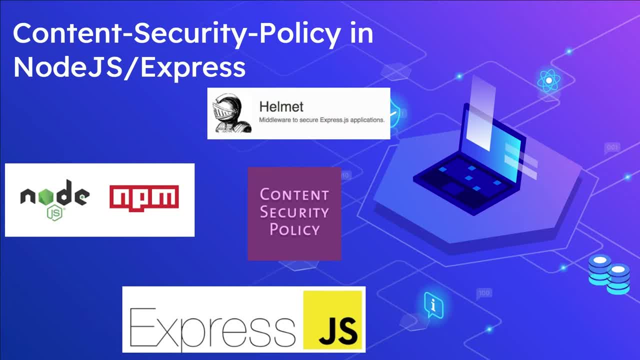 browser from which location and or which type of resources are allowed to be loaded. To define the loading behavior, the CSP specification uses directive, where a directive defines the loading behavior for a target resource type. This helps to protect against cross-site scripting attacks, XSS click jacking and other code injection attacks that rely on executing malicious content in the.